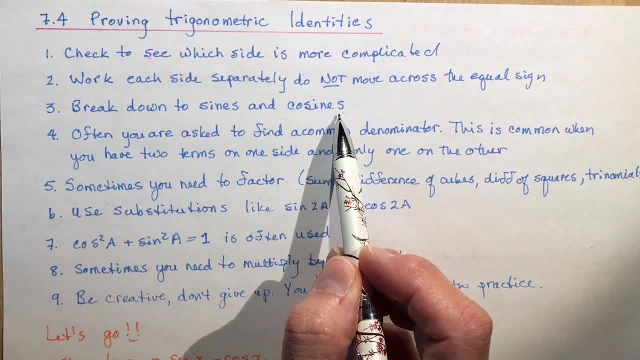 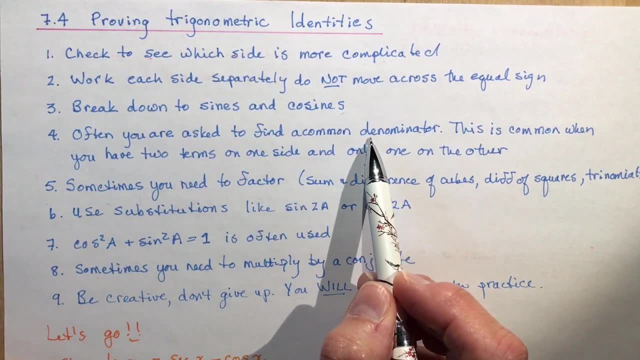 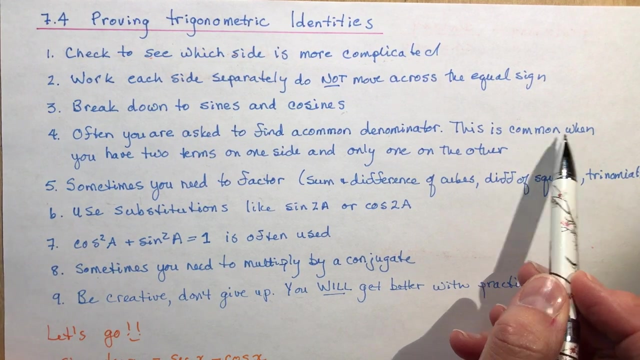 if you can break it into these little building blocks, you're more likely to see some sort of similarity. often you're asked to find a common denominator. not asked to, but you will need to find a common denominator. this is common, isn't that funny? common when you have two terms on one. 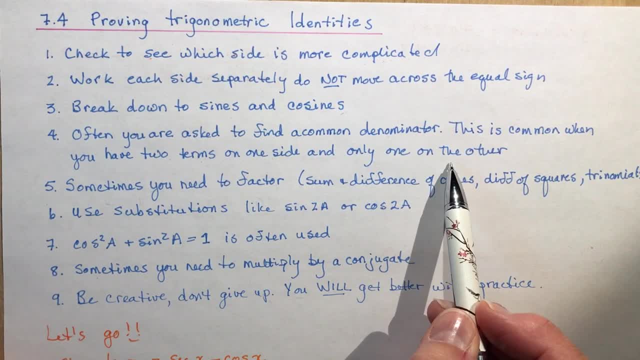 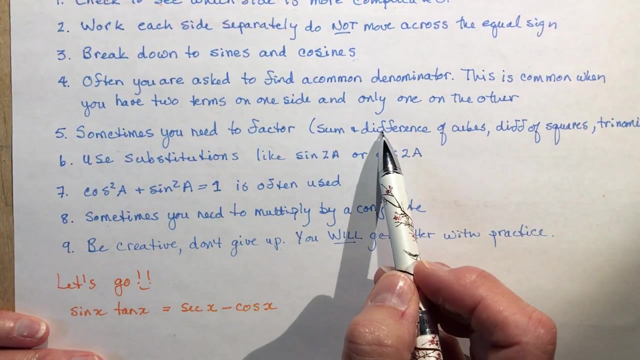 side and only one on the other. in other words, how are you going to get from having two parts to one part? well, obviously you're going to have to somehow add or subtract them together to get this one part. sometimes you need to factor, oh yeah, sum and difference of cubes, difference of squares and 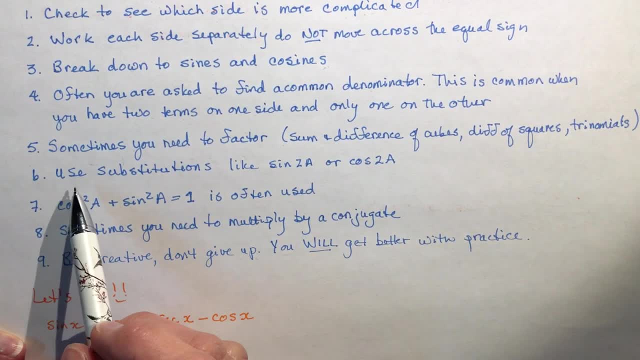 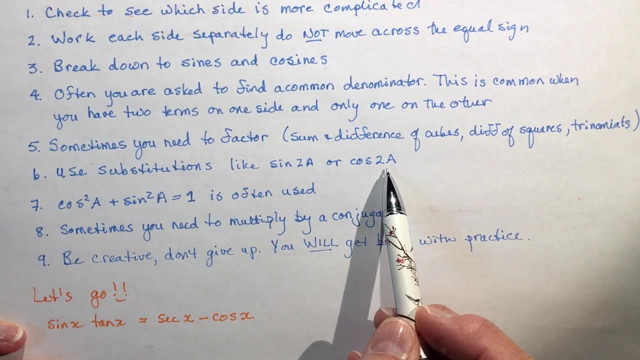 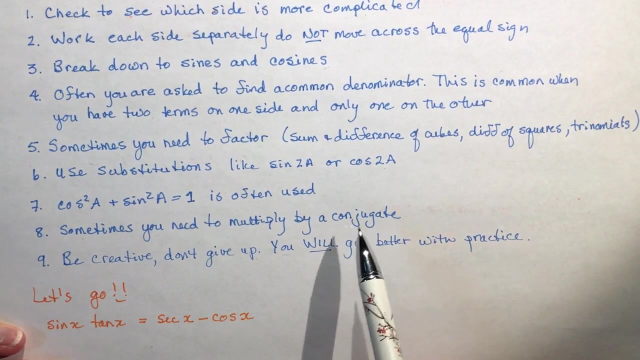 sometimes just a basic trinomial. you should use substitutions like sine 2a- that you've learned- or cos 2a. sometimes you have to expand, like the sine of x plus y. you might have to expand that using all these little tools that we've learned in the last couple of sections. cos squared, a plus sine squared equals one is often. 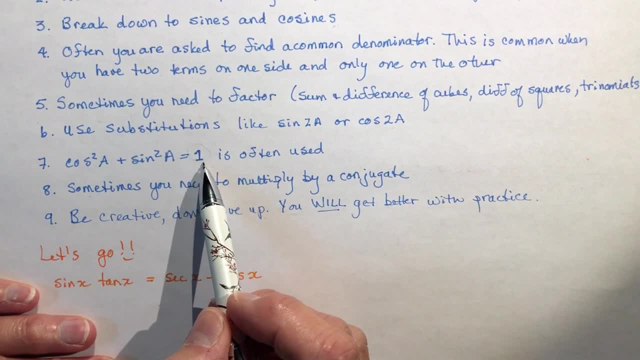 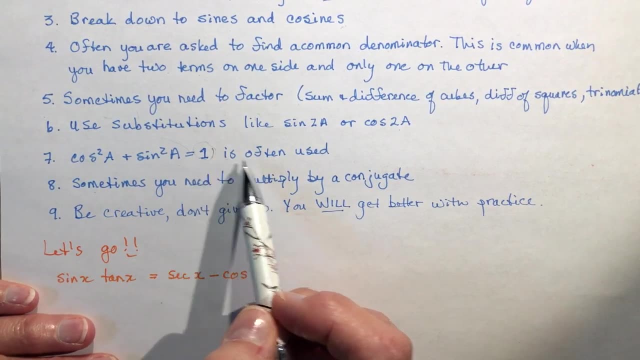 used the variations on this. you might be replacing one with this or replacing this with a one, and you'll go: oh, that was so bad, so easy. why didn't i see it? so watch out for that one. and sometimes you need to multiply by a conjugate. 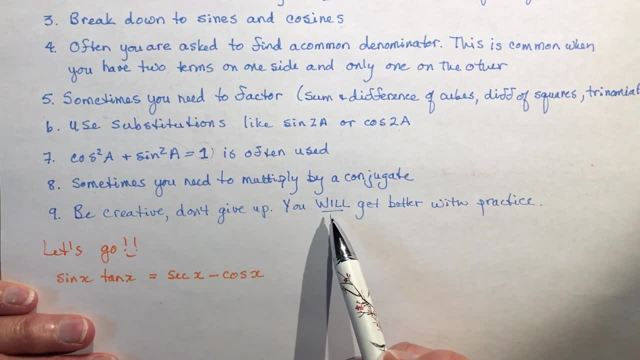 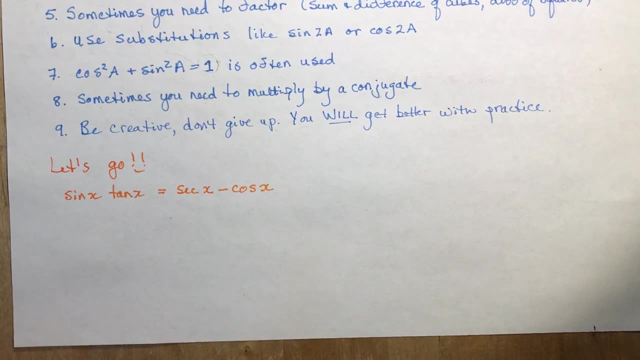 be creative, don't give up. you will get better with practice. okay, so let's go. we're going to do three or four examples and then, like i said, i will dig up some of the more difficult ones and do them for you in a follow-up lesson. so i have sine x, tan x equals secant x minus cos x. well, they both. 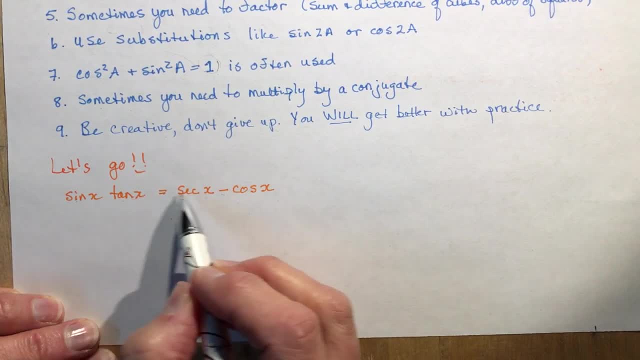 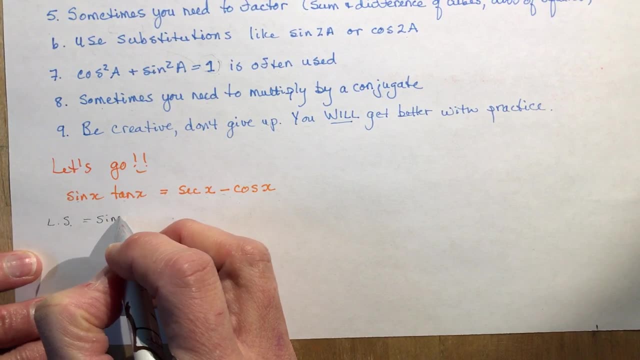 have something that i can break down. this one is all one part, this is two parts, so i'm thinking of those things as i do them, and don't forget to look from left to right as you're working with it to see what direction you should be going. 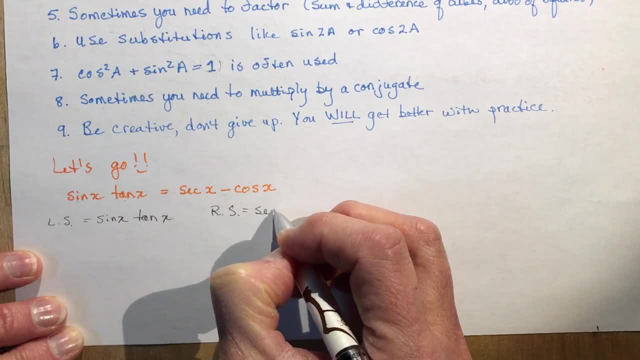 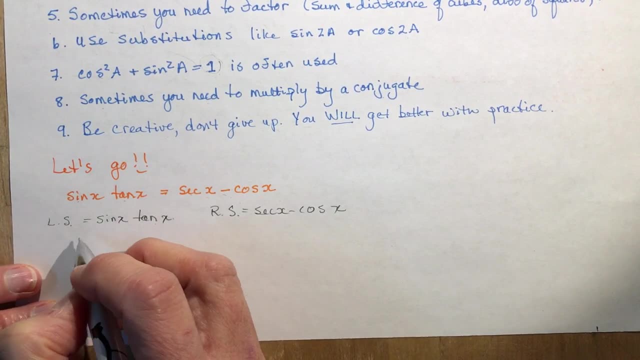 in. so i'm going to write what the left side is, what the right side is, and then i'm going to start simplifying. okay, so i know that tan x is sine x over cos x, so i'm going to replace that, always replace tan or a reciprocal��ned一个. 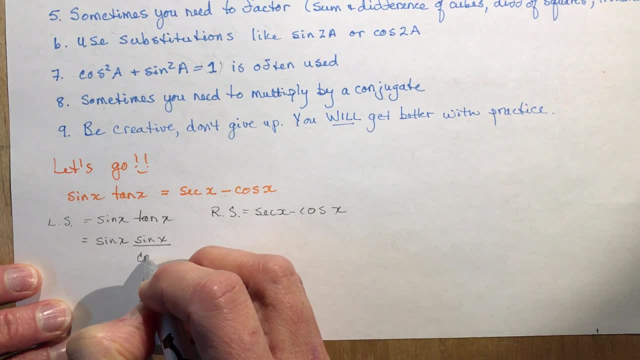 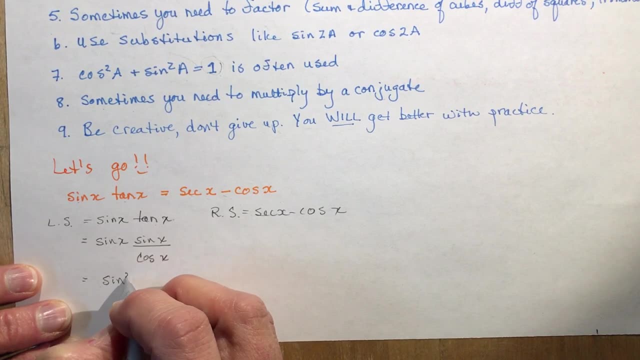 or a reciprocal 부47xということ to另一个. function by the sine and cosine. so now I have sine x times sine x. oh, that would just be sine squared x, isn't it over cos x. okay, let's just run over to the right side here for a minute to see. 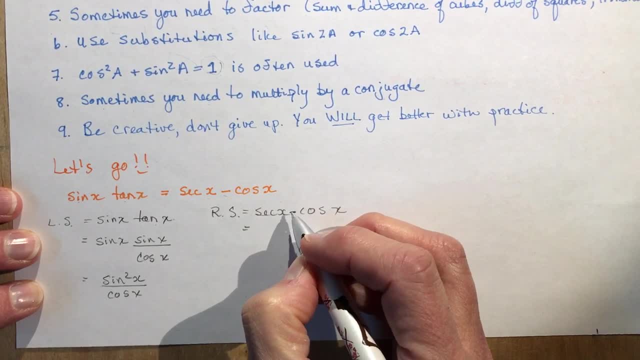 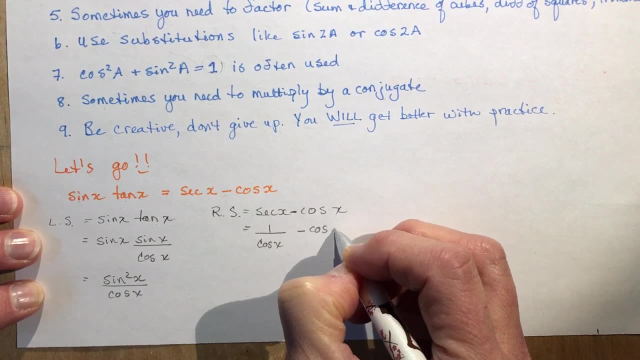 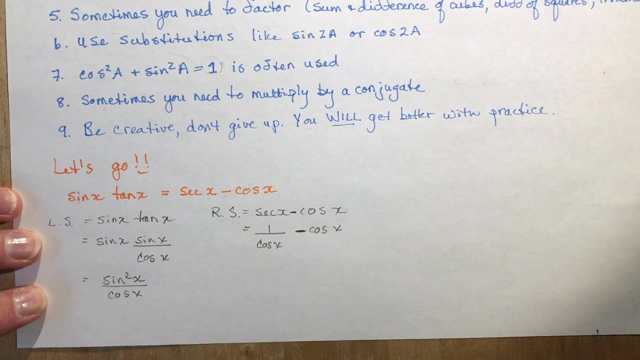 what we've got here. we have a minus sign here. so what's secant? secant is one over cos right, one over cos x minus cos x. so I see how I have only one term on this side and I have two things here. so that means I'm going to find a common denominator here, which of course, is going to 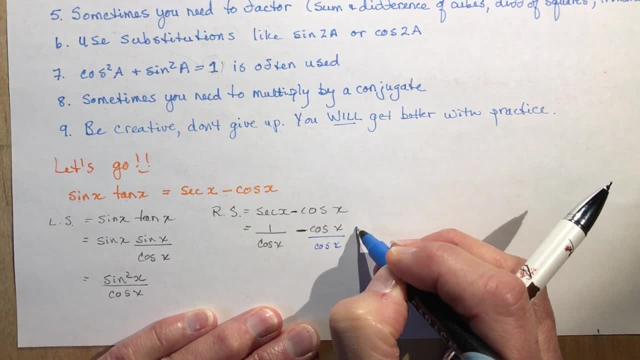 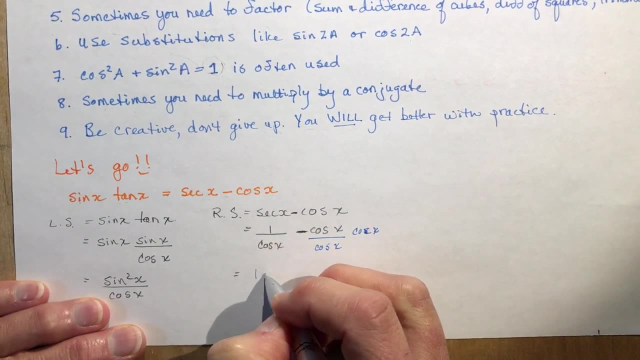 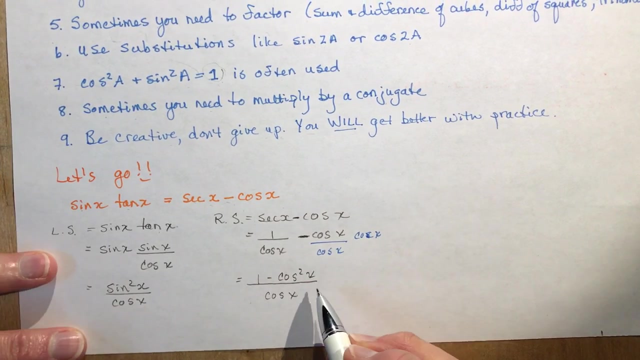 be cos x. so I'm going to multiply by cos x over cos x, oops cos x, and that's going to give me one minus cos squared x all over cos x. and oh gee, isn't one minus cos squared x the same as sine squared x? so there we go. 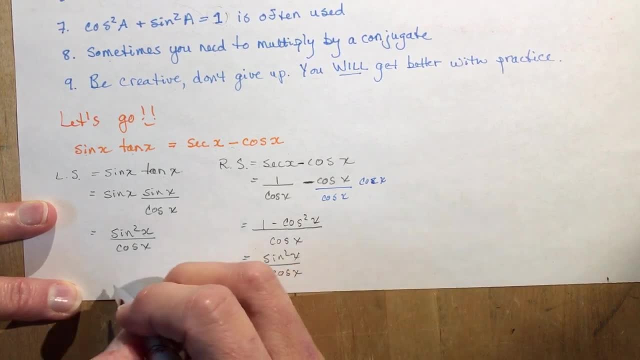 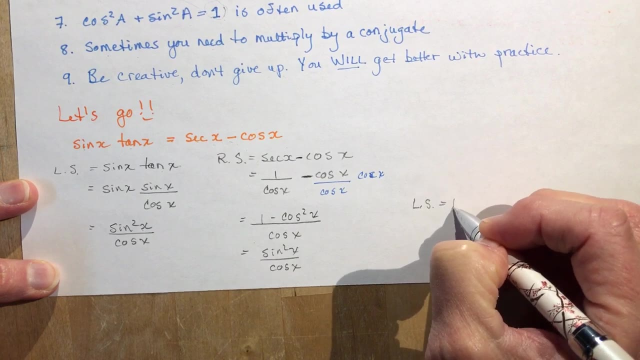 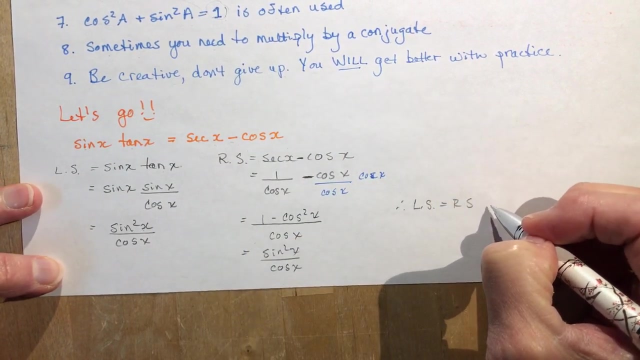 now I don't know what your teacher asked you to write once you're finished. in my class I would have had them just say left side equals right side, and you can either rewrite this saying that they're equal. I also used to get my students to write QED. 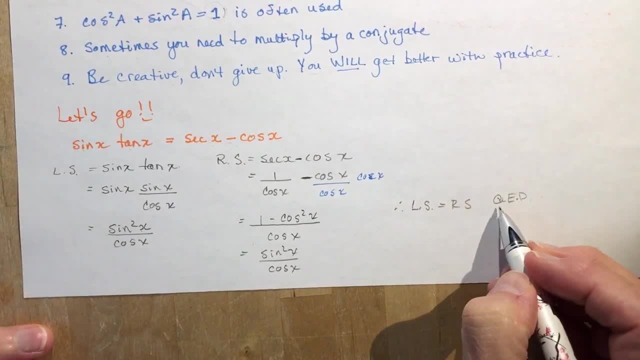 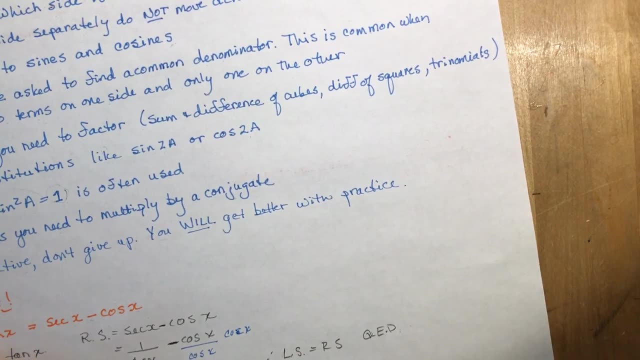 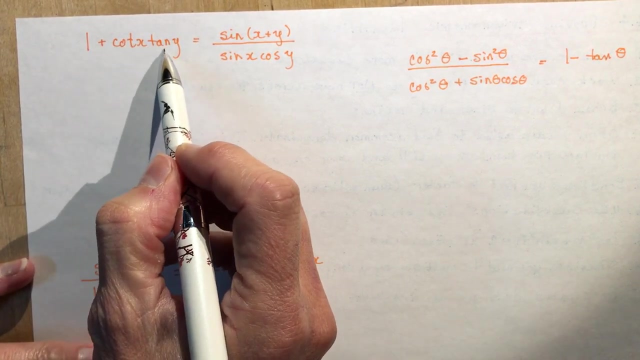 which means quadratus, quad, eratostem and stratum. Therefore it has been proven. Maybe you want to see if your teacher will let you get away with that quick little short form. Okay, so let's flip over and look at something a little more complicated. So here I have 1 plus coten x. tan y equals sine look. 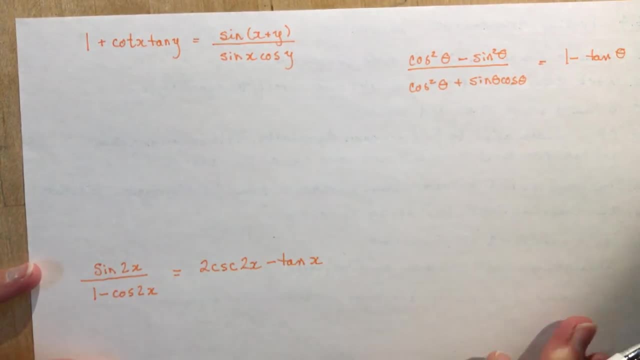 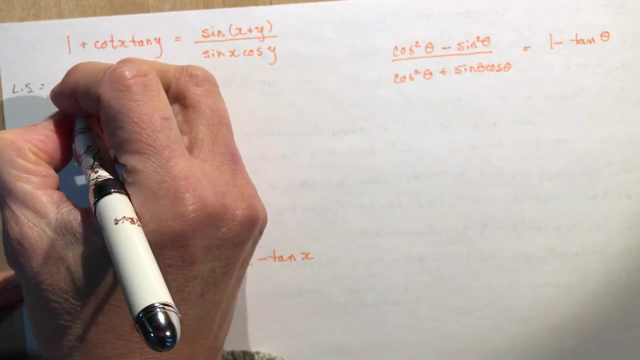 x plus y. Well, we just learned how to do that, So you're going to be able to break that up. And well, let's just start with the left side. So I have 1 plus coten x, tan x, sorry, tan y. 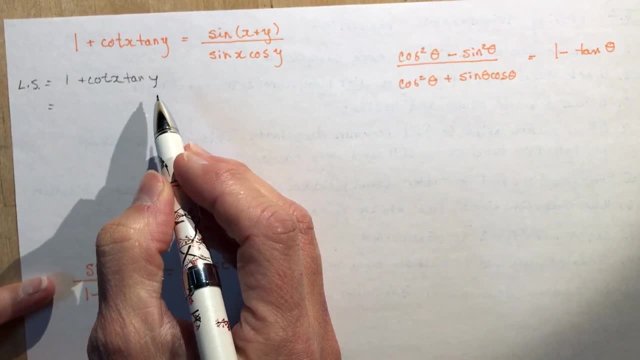 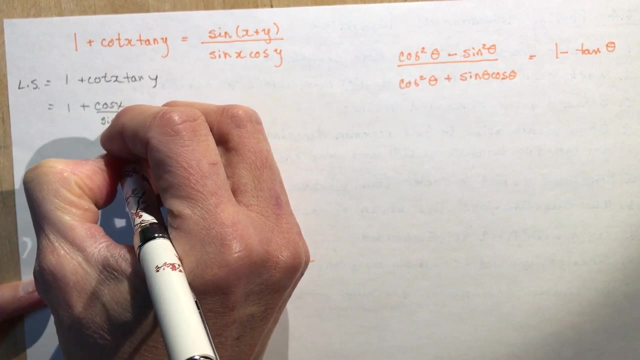 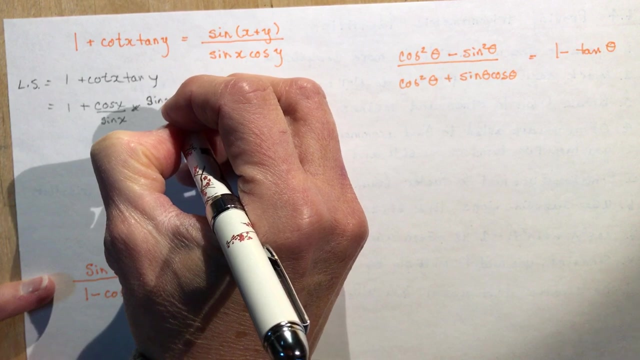 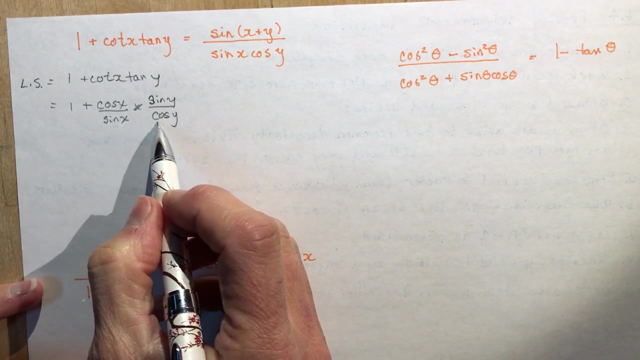 And I know that coten x now break it into sines and cosines, right? So coten is cos x over sine x and tan y, and it's multiplied here, So I have sine y over cos x Y. Okay, now, when I'm at this point, I just keep looking over here and notice how this 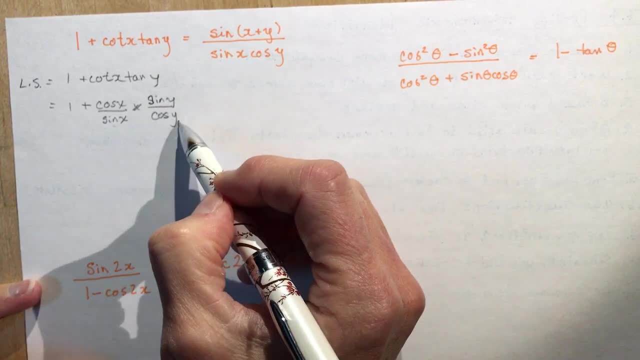 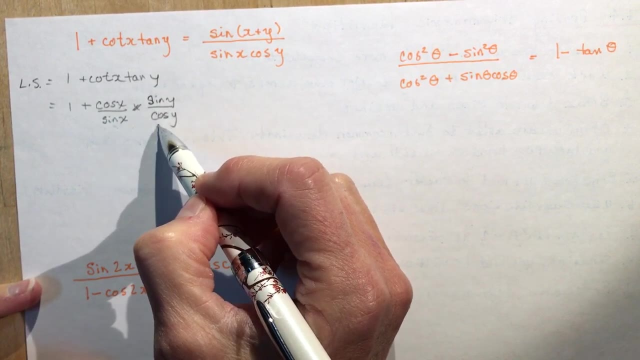 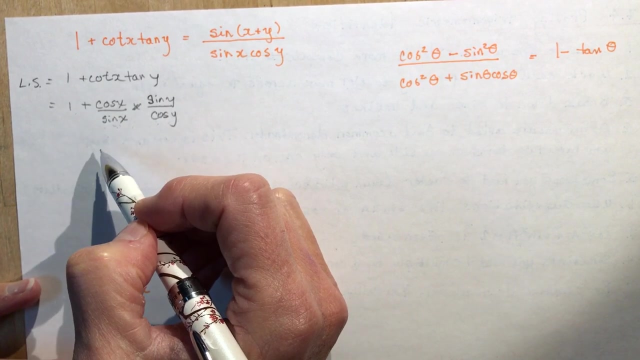 denominator is already sine x- cos y, which I would have here, right, If I just multiplied these. So I have cos x sine y over sine x cos y, and I have a 1.. So I'm either going to do something with that 1, or I'm going to. well, what I'm going to do now is I'm just going to. 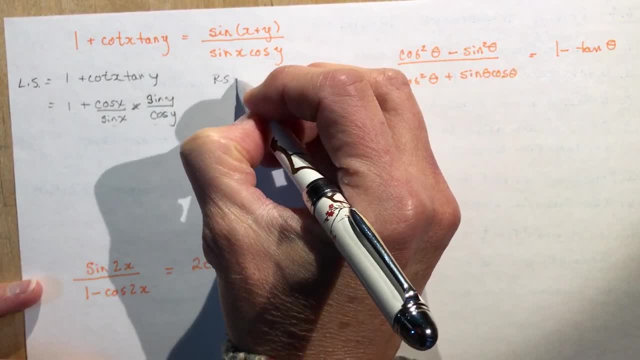 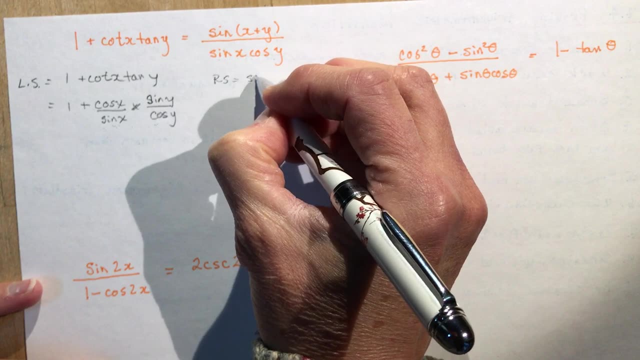 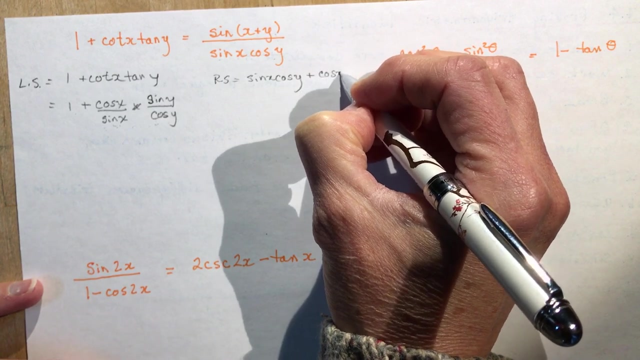 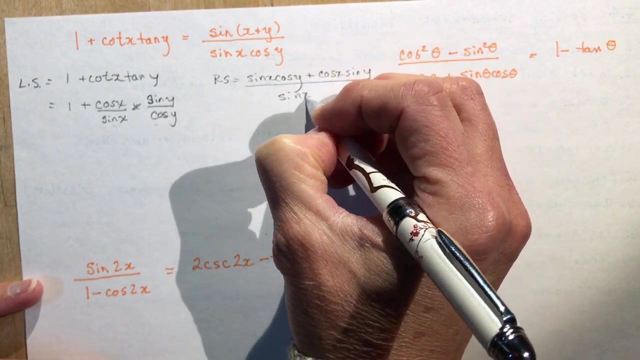 I'm going to. we're going to startais going to leave this side and run over here, because the right side was pretty complicated with this addition formula. So sine of x plus y, remember, is sine x, cos y plus cos x sine y, and that's all over. 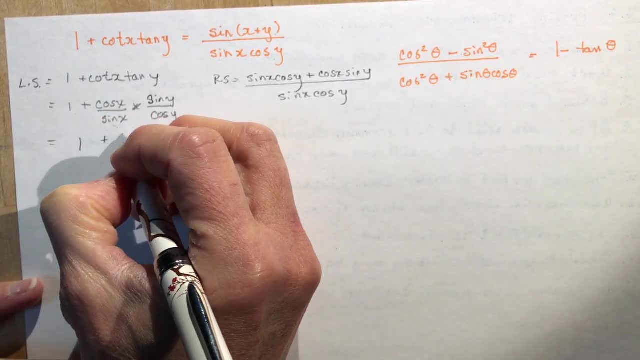 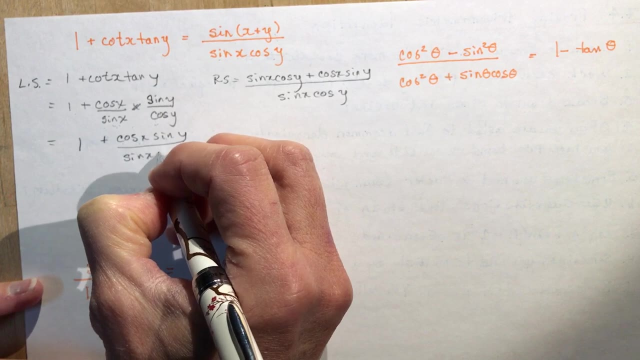 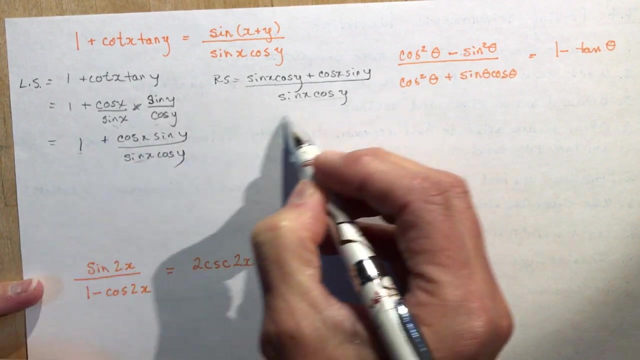 sine x cos y. Note the other side here. I'm just going to write this like this: first, cos x sine y over sine x cos y and I'm going to compare what's the same here. Well, I've got the right denominator, but I have this one here and I have this, so look. 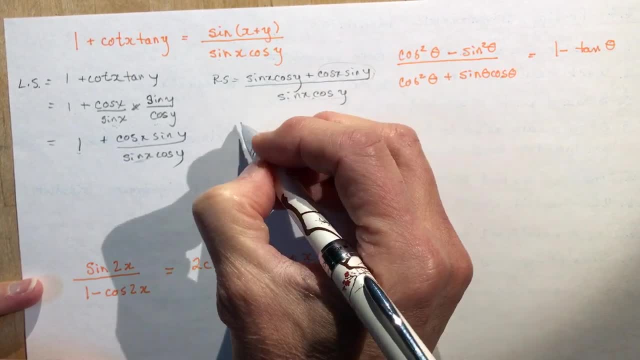 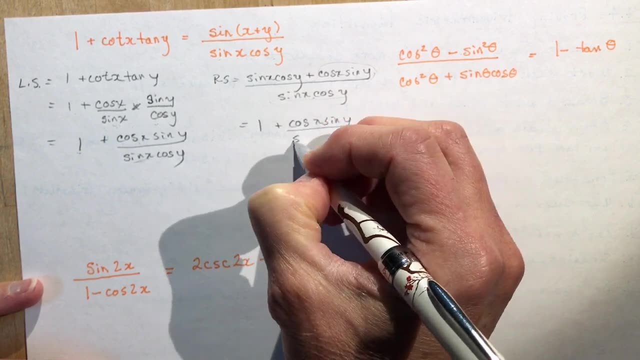 that's like this and this one over, this is a one right, so I have what I need here. Let me just show you how I got that, in case you're saying: how did you make a one out of that? I know some of you are saying that I can hear you. Okay, so if I 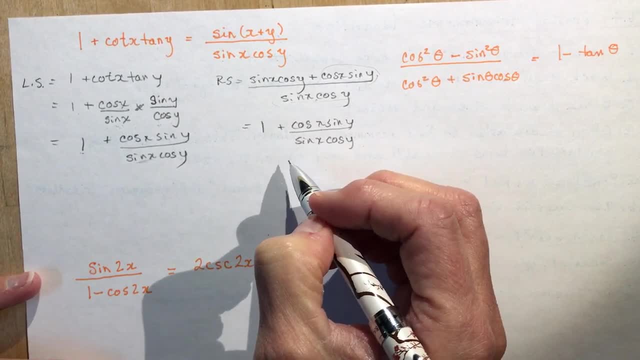 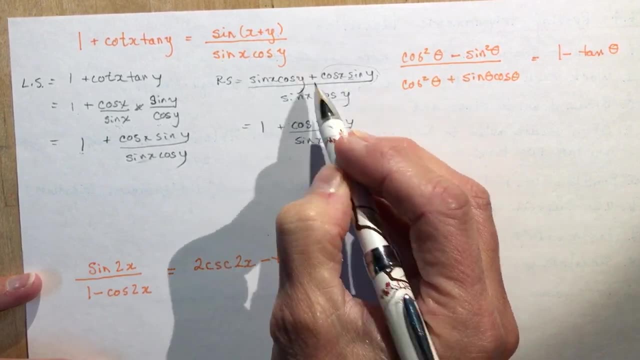 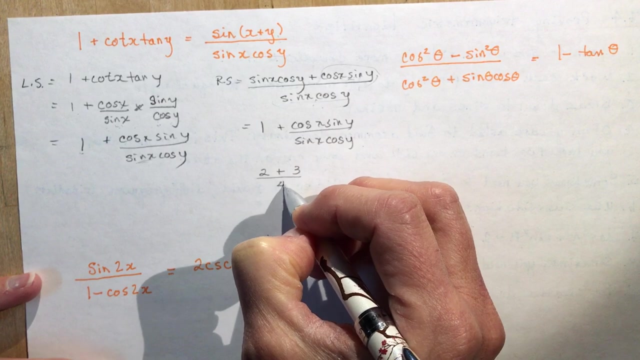 had something like this, and always I always tell my students to think of a really basic, simple equation. if you're not sure what to do When I have something added together over a common denominator, it's like me saying: if I had 2 plus 3 over 4, okay, so say this was 2, this was 3, this was 4, that's the same as. 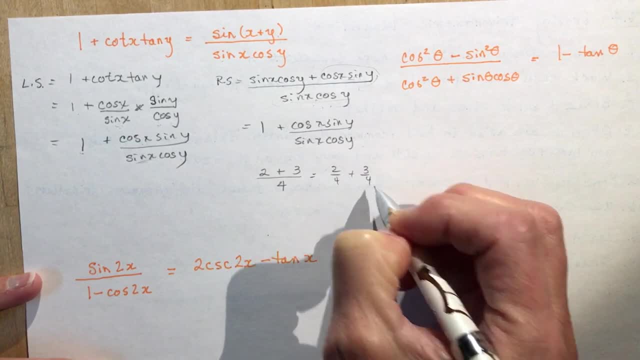 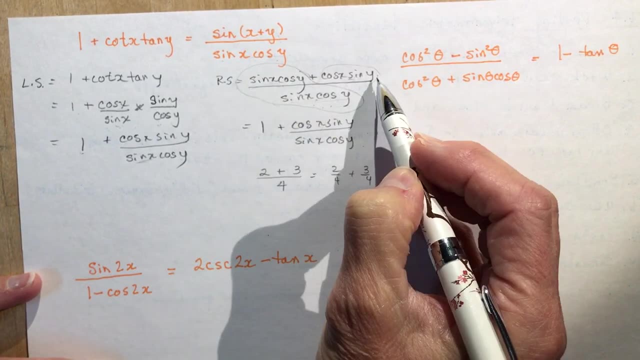 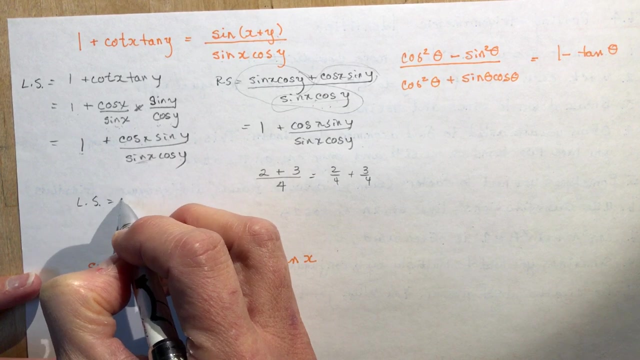 2 over 4.. 4 plus 3 over 4.. So that's what I've done here. I've broken this, so I have this one which becomes the one, and I have this one which is still this. So now I have left side equals right side, for left side equals right side, QED, and that's. 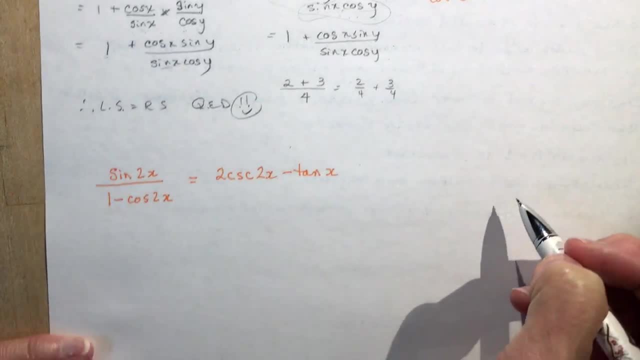 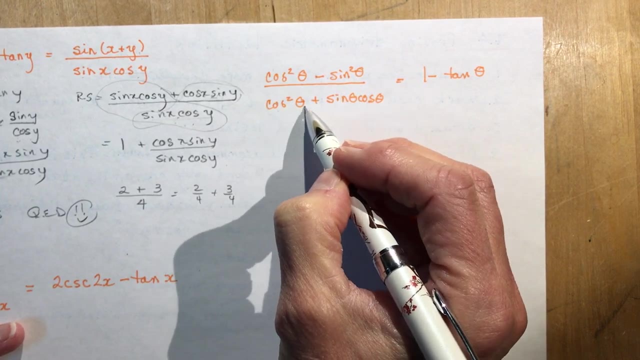 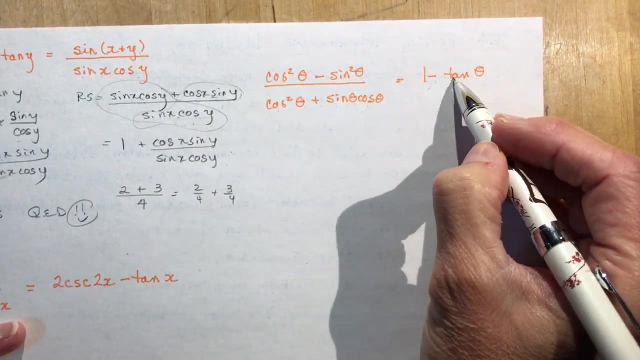 always nice to write after it too. It will help your face. Okay, let's go down. oh, let's do this one here: cos squared theta minus sine squared theta? cos squared theta plus sine theta? cosine equals 1 minus tan theta. Obviously, this is a more difficult one, but this tan can be broken down into. 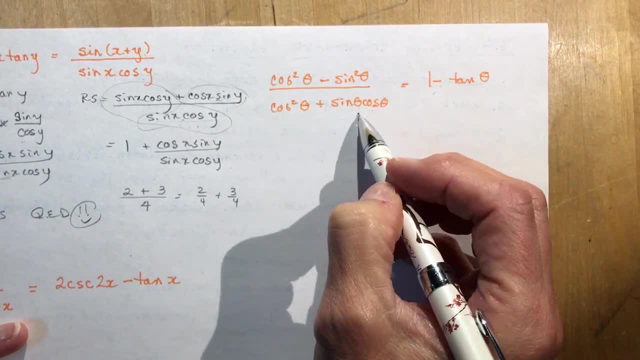 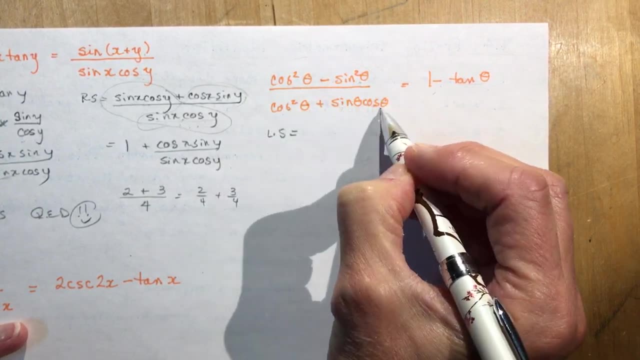 sines and cosines, Because we have lots of those here. that's probably what we're going to need to do. So with the left side here, I can see that these all have some factoring skills that I could use for them. right Cos squared minus sine. 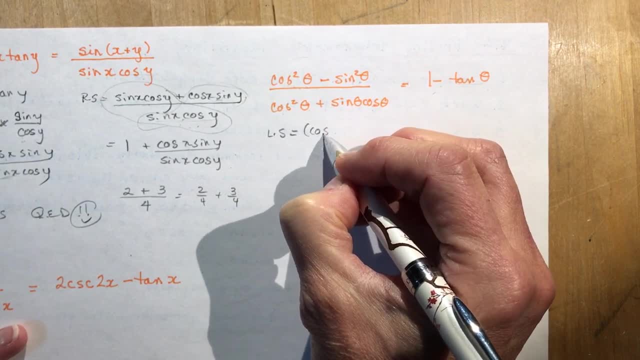 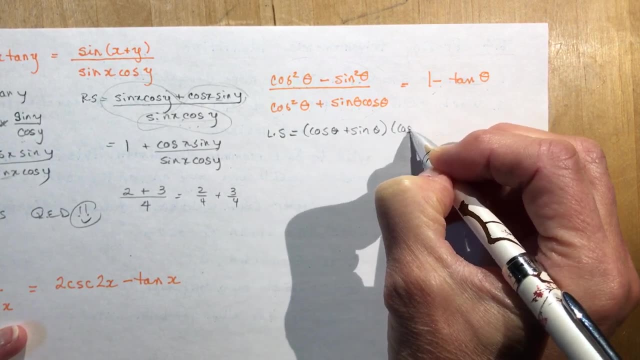 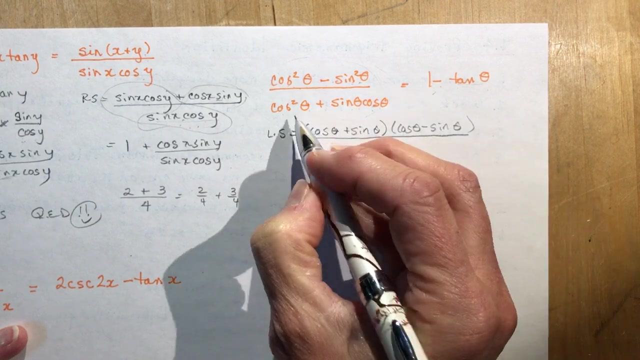 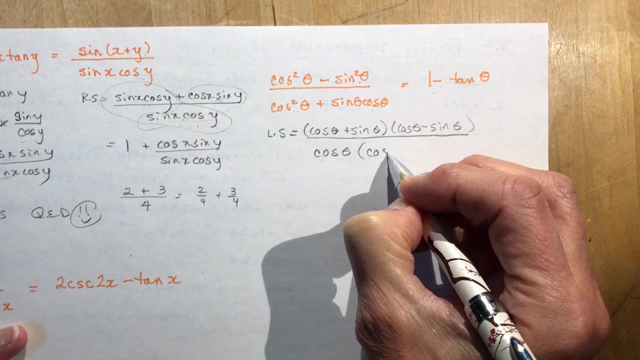 squared. that's a difference of squares. So I'm going to say cos theta plus sine theta times cos theta minus sine theta. Oh, I took up more space than I wanted to And in the denominator I have a common factor. right, I can take out a cos theta. What am I left with? Cos theta plus sine. 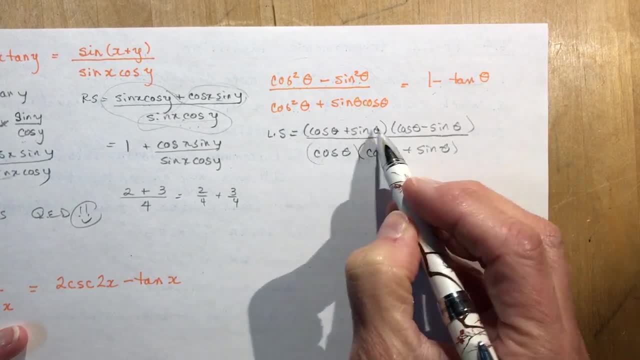 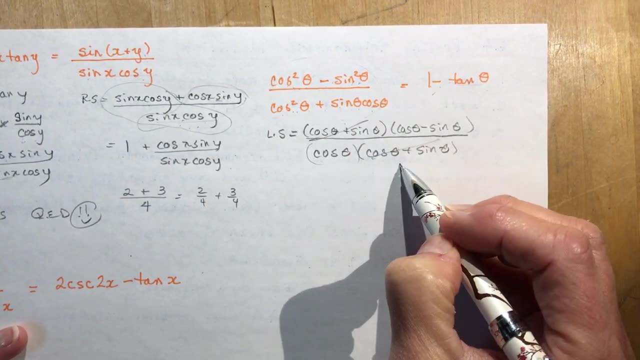 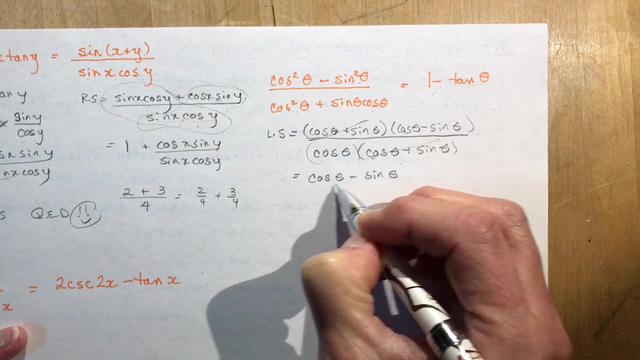 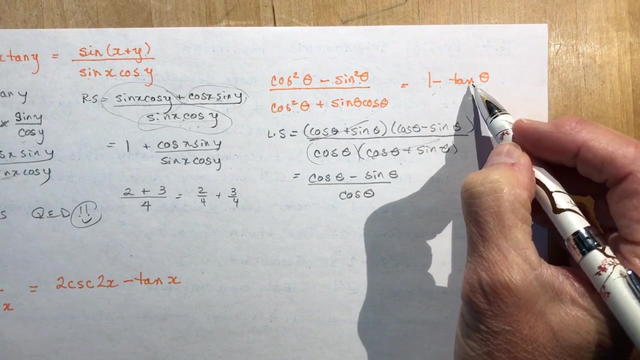 theta. Now all these things are multiplied together. right, and once things are multiplied together, you can cancel them out, as little packages Divide into each other, and that leaves me with cos theta minus sine theta over cos theta. Now you can go over to the right side here and break this down. but I'm looking at this and I already 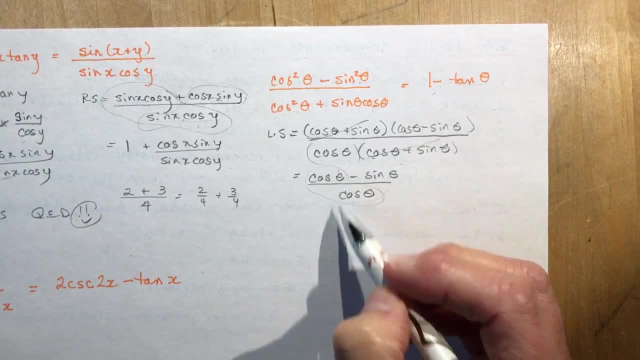 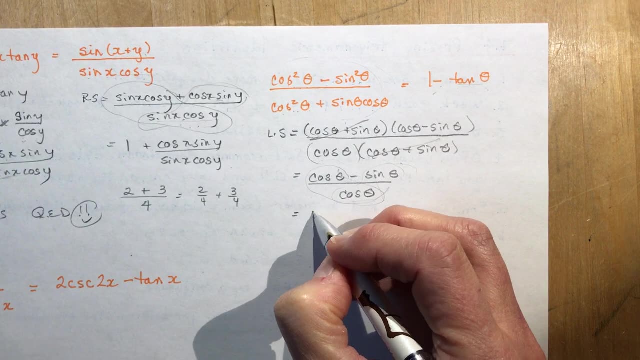 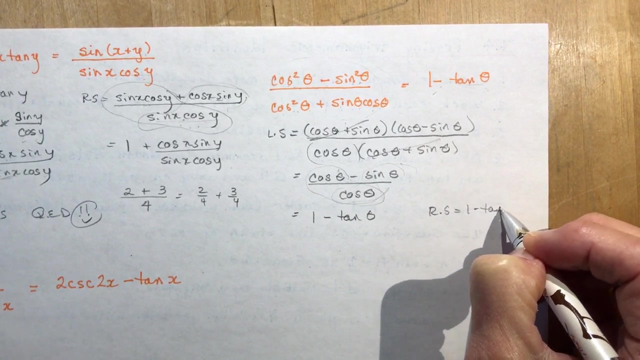 see that answer, Do you? Because look cos theta over cos theta, that's 1, and sine theta over cos theta is tan theta. So I would just say: oh, this is equal to 1 minus tan theta, and right side equals 1 minus tan theta. So therefore left side equals right side. and a little tricky. 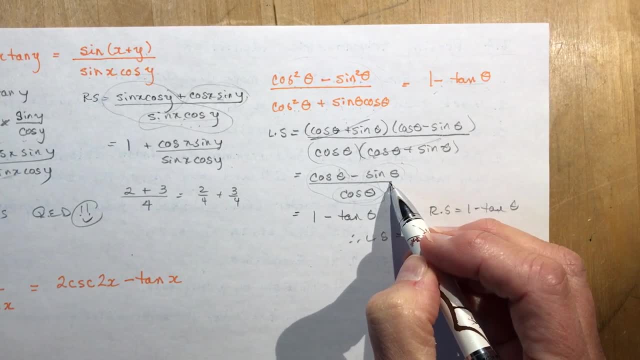 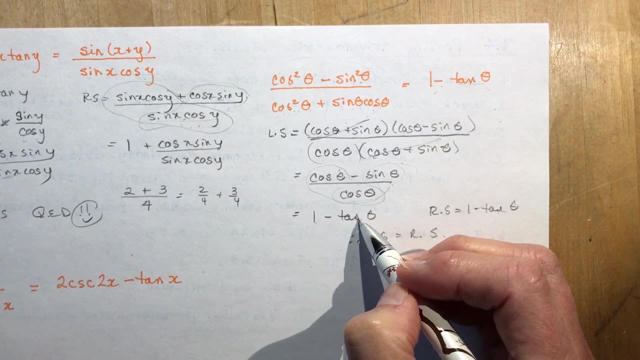 thing. if you get to here and sometimes don't, don't tell your teacher, I told you this. but if you just jump and say, oh, that's equal to this, even if you're not sure, and say left side, right side, she's going to think you knew that. 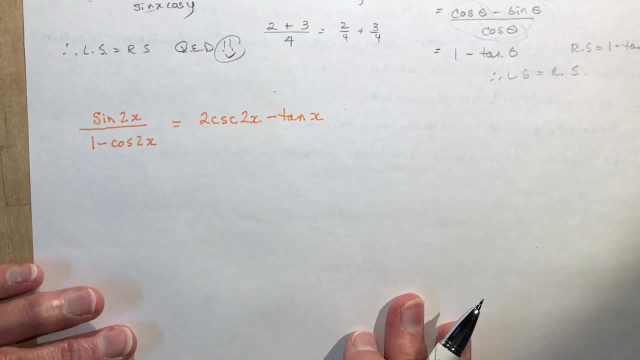 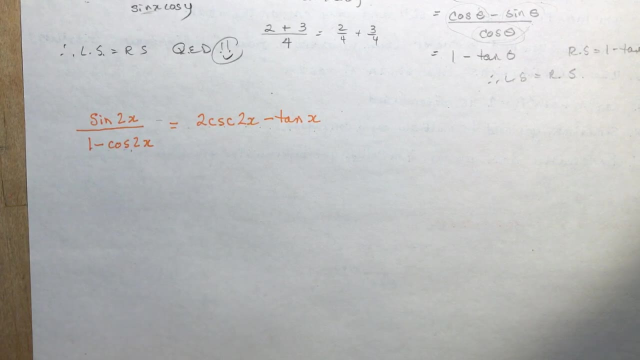 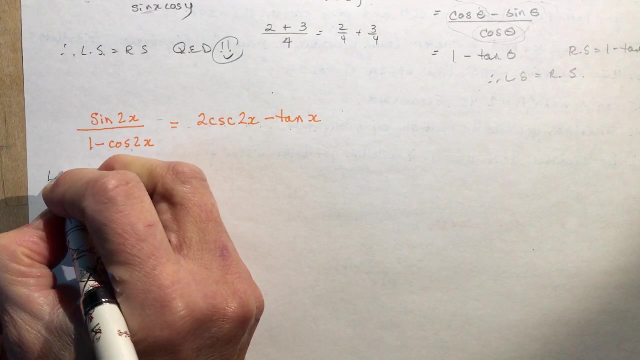 But you should write it down Right. Ok, last one: Sine 2x 1 minus cos 2x equals 2 cosecant 2x minus tan x. Ooothat one looks really complicated, doesn't it? Ok, so let's see what can we do with the left side Sine of 2x. Well, the 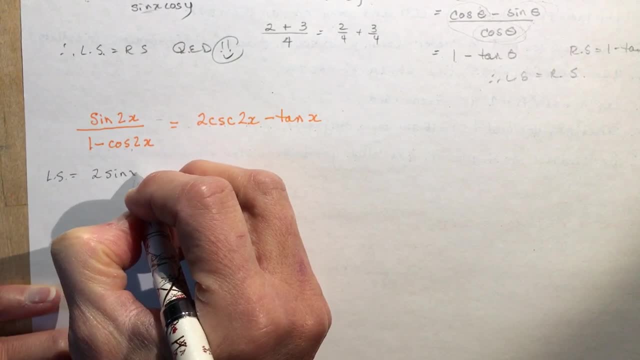 sine of 2x is 2 sine x cos x. And I'm all over cosine 2x. Ah, I forgot that Sine of 2x is 2 sin cos x. Off the top's and I move my clusters side. 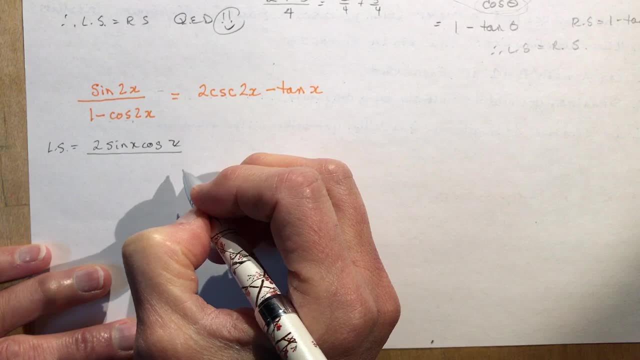 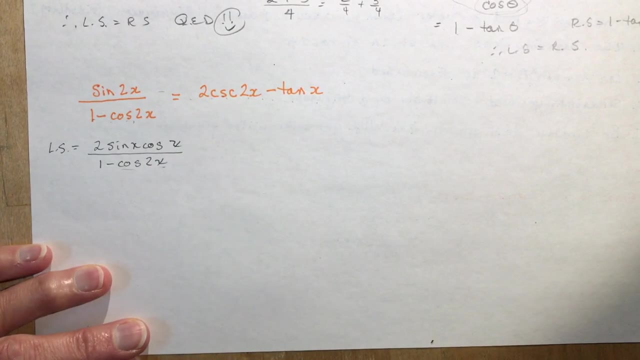 Ok, Sine of 2x, 1 minus cos 2x. I'm going to write that down here anyway, even though I know I'm going to want to change this cos of 2x. Let's go to the right side just to see what kind of denominator I want. 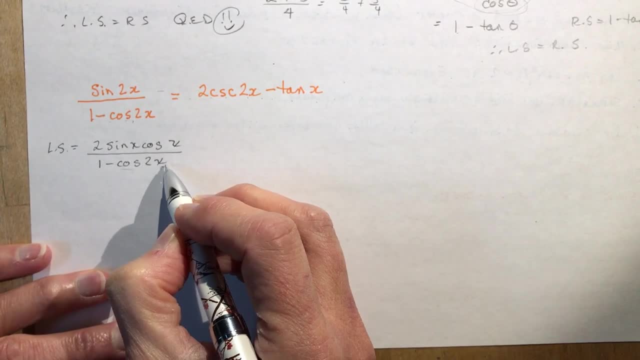 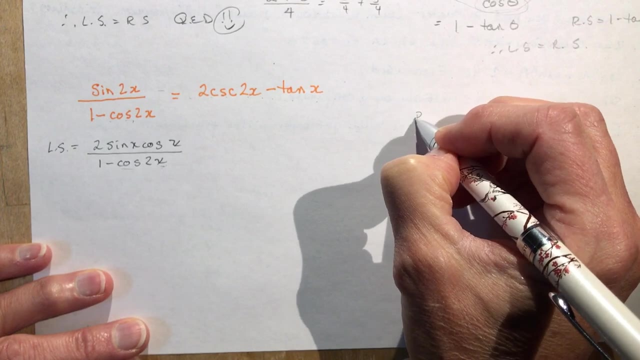 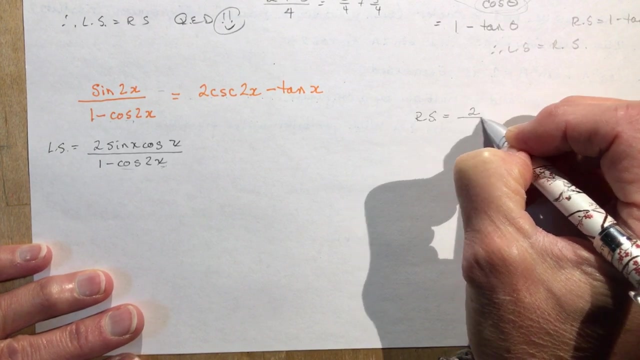 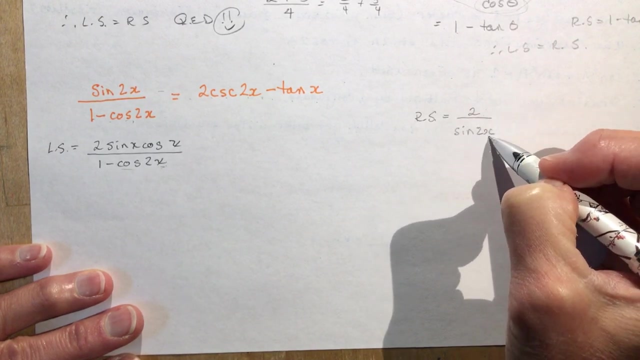 because, as you know, the cos of 2x has three possible equations that I can substitute in here. So I'm going to go to the right side first. I'm going to put it right over way over here: So 2 cosecant 2x, that's 2 over cosecant 2x is 1 over the sine of 2x, So I have 2 over sine 2x. 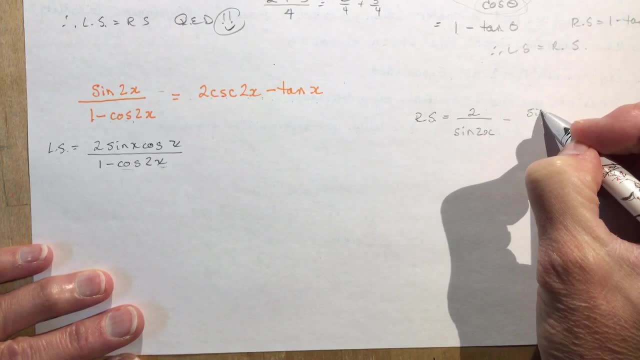 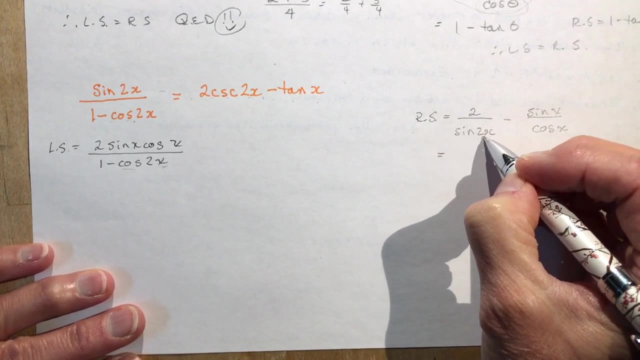 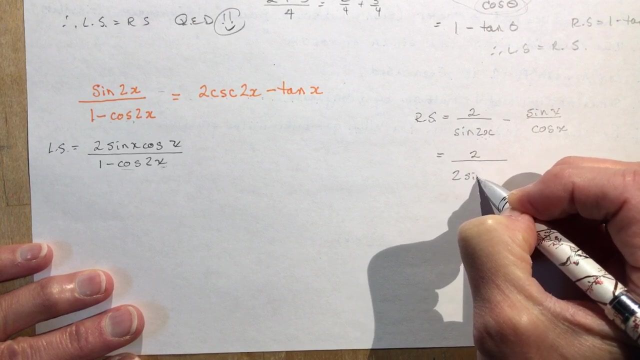 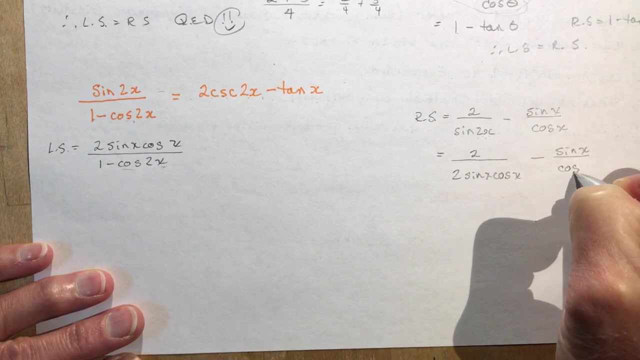 and the tan x is going to be sine x over cos x. Now there's only one identity for sine of 2x and that's 2 sine x, cos x. So I'm going to write that here: 2 sine x, cos x, minus sine x over cos x, And you can see well, these twos will cancel into each. 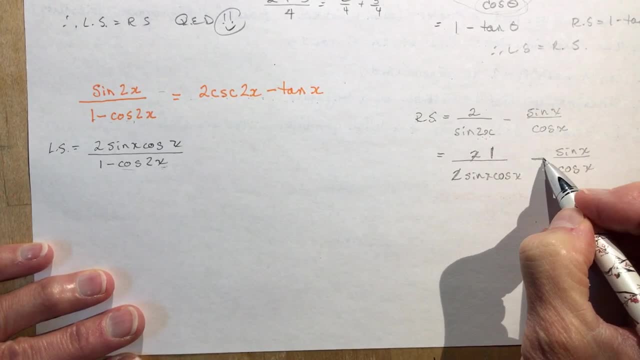 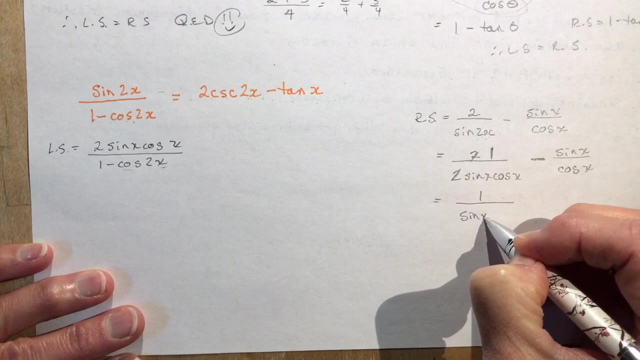 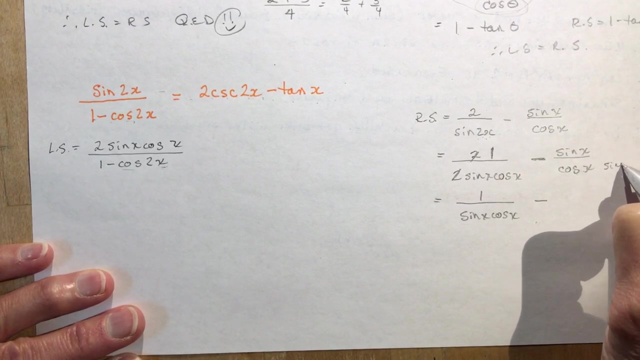 other and I have a 1 up here, And to subtract these from each other I need a common denominator. So I'm going to write this as 1 over sine x, cos x minus. now that means I have to multiply this side by sine x. 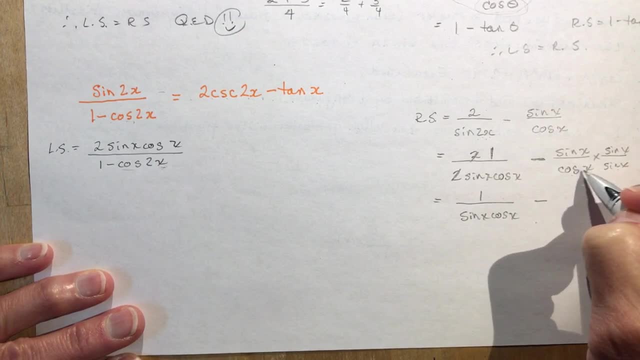 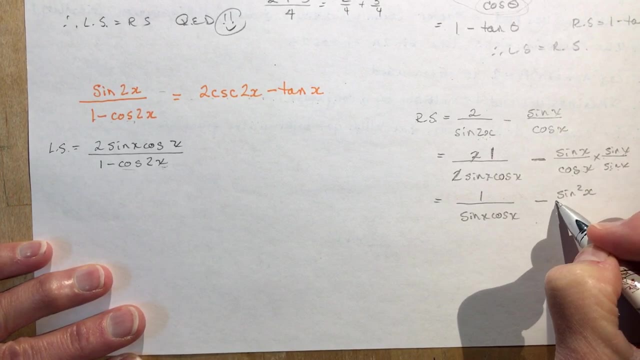 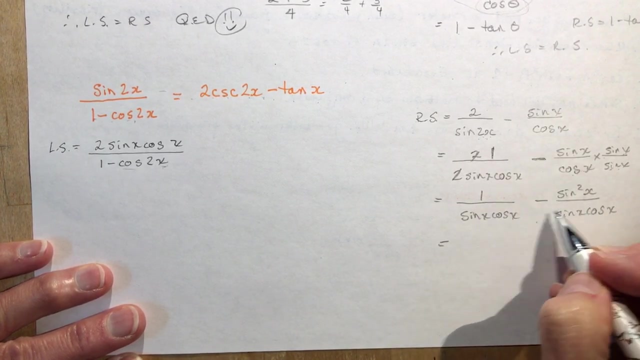 So I'm going to write this as 1 over sine x, right common denominator. So if I do that, I'm going to have sine squared x sine x times sine x over sine x cos x, And that means this one's going really well, isn't it? it's easy to see what you can do with this. 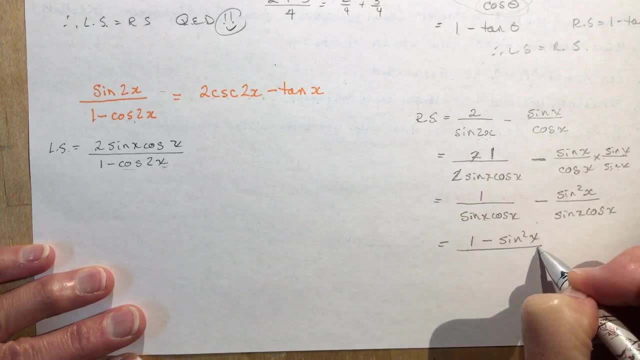 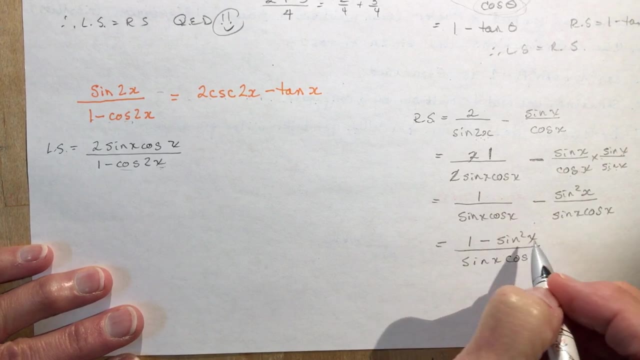 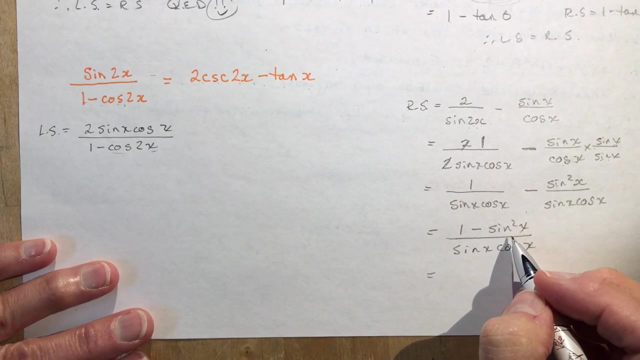 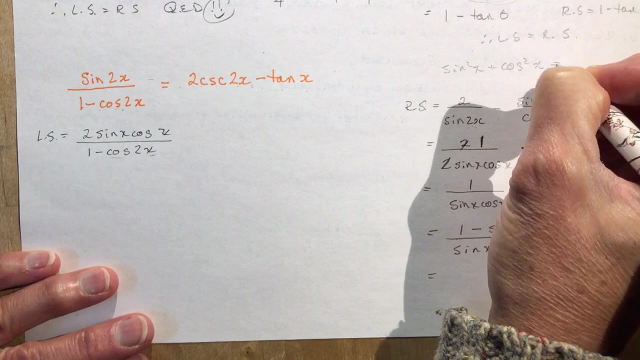 I have 1 minus sine squared x over sine x, cos x x. and what's one minus sine squared x? well, that's just co-squared x, isn't it one minus sine squared x? remember, we had sine squared x plus co-squared x: equals one. 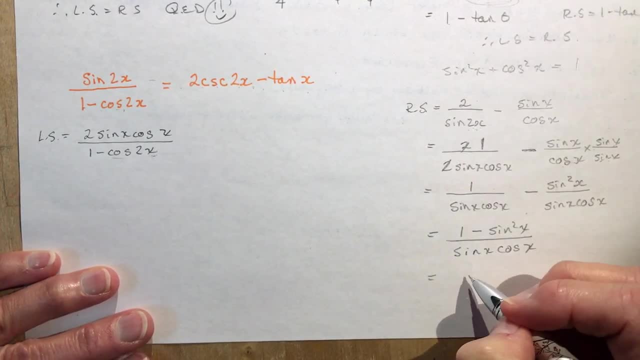 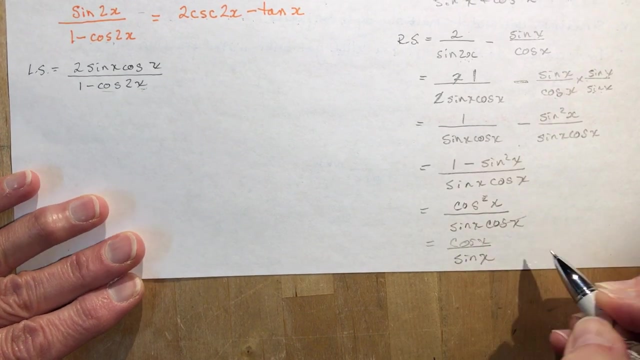 so one minus sine squared x is co-squared x, so i have co-squared x. sometimes they just flow so nicely, don't they? you're probably going- come on, ms harratt, this is painful, okay. so i have a co-squared over a cos that's going to get rid of the squared, and i have cos x over sine x. okay, now you could. 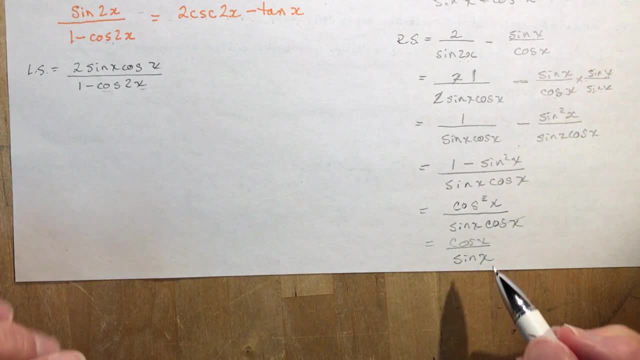 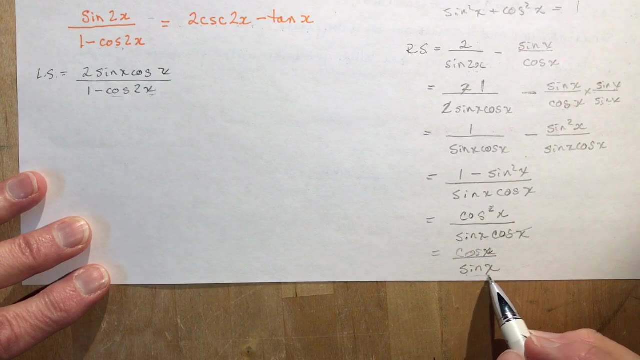 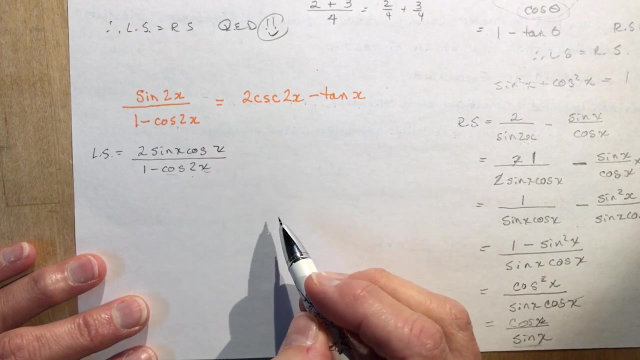 say, well, that's just cotan x, but we're not going to go there because we've got it nicely into sines and cosines, okay. so if you look here now you see my denominator is sine x and i have cos 2x here. so remember that one of the formulas you could use for cos 2x, that was one. 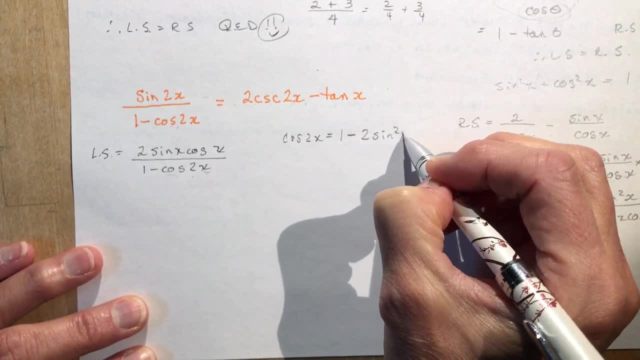 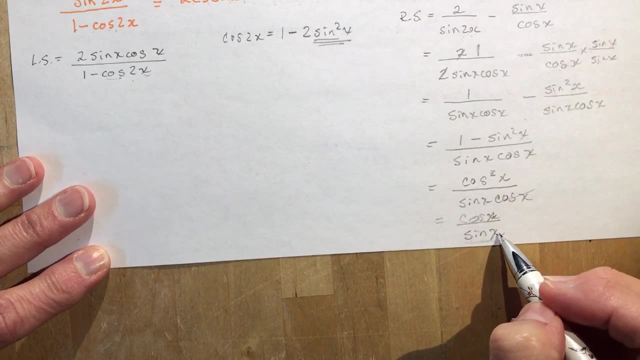 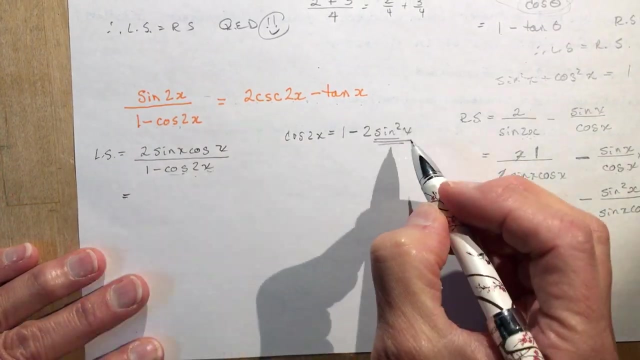 minus two sine squared x, and that will bring in a sine x into the denominator, which is what i really want to have, like i do here, because i want i want to get this to be cos over sine. so i'm going to substitute the cos 2x with the cos 2x and i'm going to substitute the cos 2x with the cos 2x. 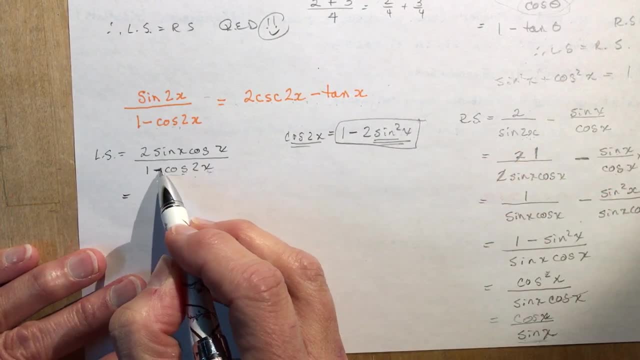 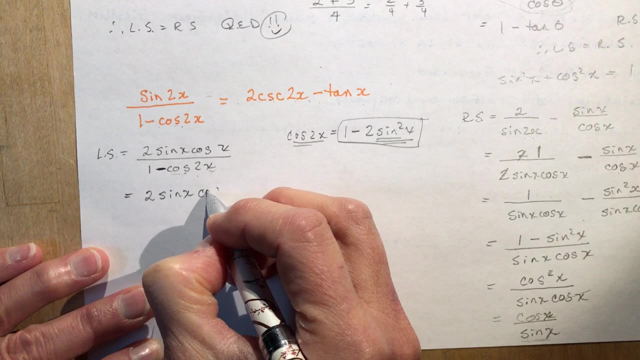 and i have cos 2x here, so remember that one of the formulas you could use for cos 2x, that was one with this. don't forget the whole part. and don't forget this minus sign. remember most of the mistakes in math are made because of negatives. whoops, got something under the paper there.